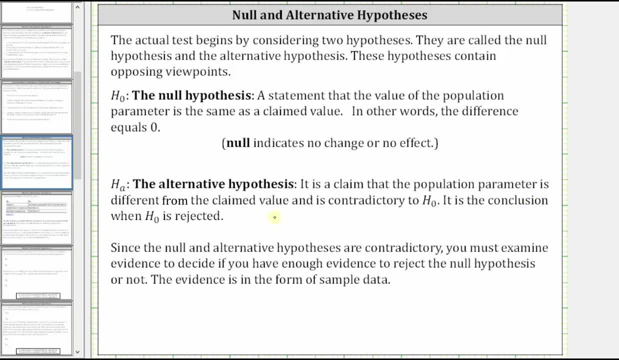 is a claim that the population parameter is different from the claimed value and is contradictory to H sub zero, the null hypothesis. It is the conclusion when the null hypothesis is rejected. Since the null and alternative hypotheses are contradictory, you must examine evidence to determine. 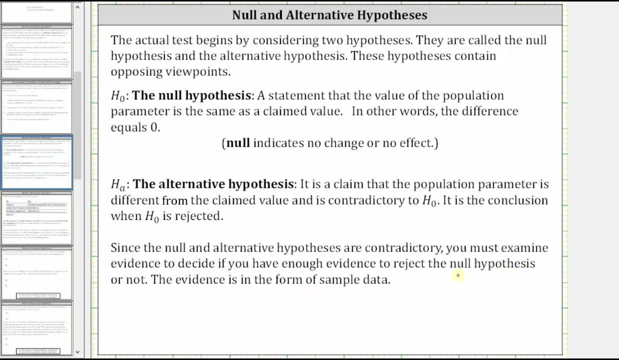 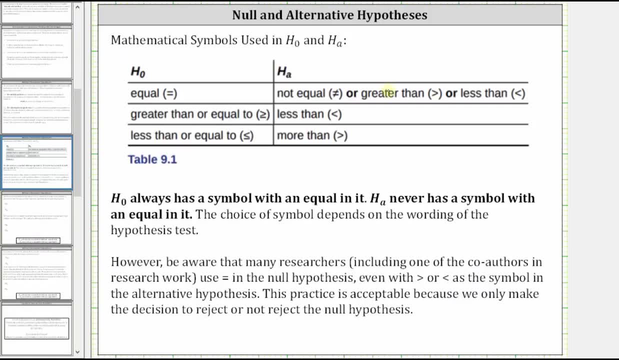 if you have enough evidence to reject the null hypothesis or not. The evidence is in the form, in the form of sample data. Looking at the table, notice how the mathematical symbols used for the null hypothesis are equals, greater than or equal to, or less than or equal to. 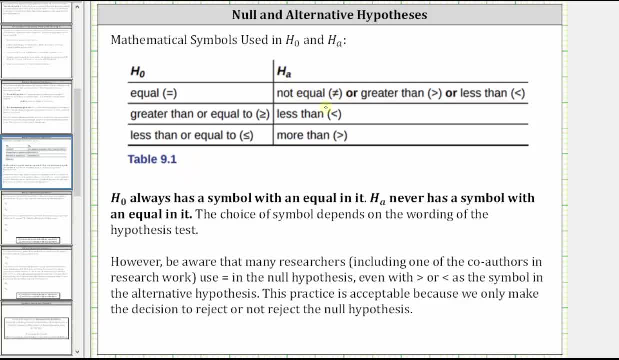 For the alternative hypothesis, so H sub zero. the null hypothesis always has a symbol with an equal in it. The alternative hypothesis never has a symbol with an equal in it. The choice of symbol depends on the wording of the hypothesis test. However, it is important to recognize 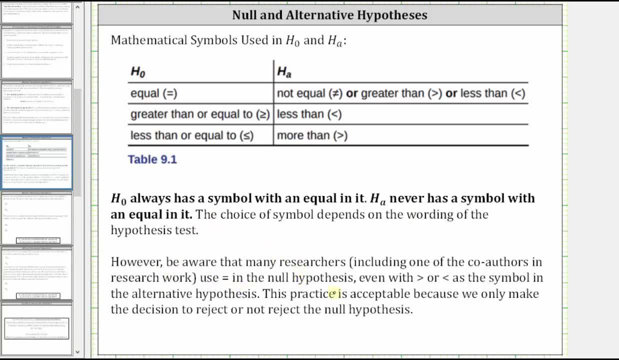 that many researchers use equals in the null hypothesis, even with greater than or less than as the symbol in the alternative hypothesis. This practice is acceptable because we only make the decision to reject or not reject the null hypothesis, So in that case you wouldn't see greater than or equal to. 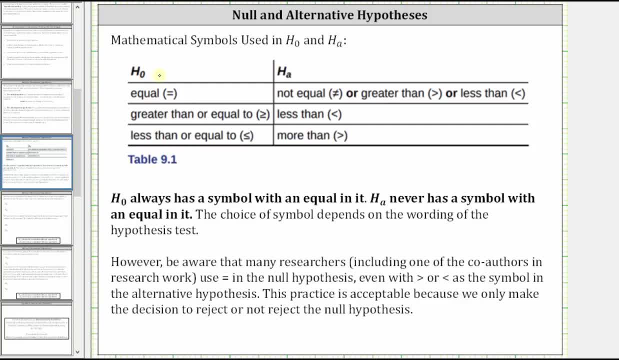 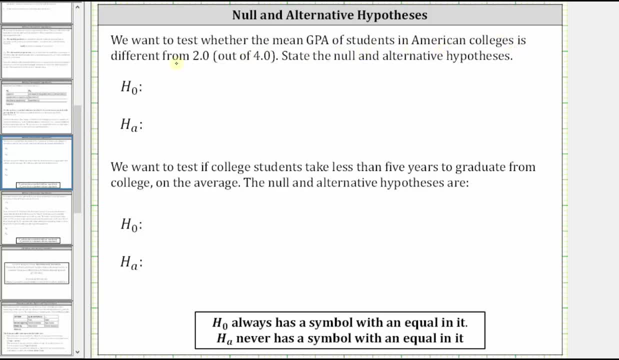 or less than or equal to in the null hypothesis. Let's take a look at some examples. We want to test whether the mean GPA of students in American colleges is different from 2.0, state the null and alternative hypotheses. So we're trying to test to see whether the GPA 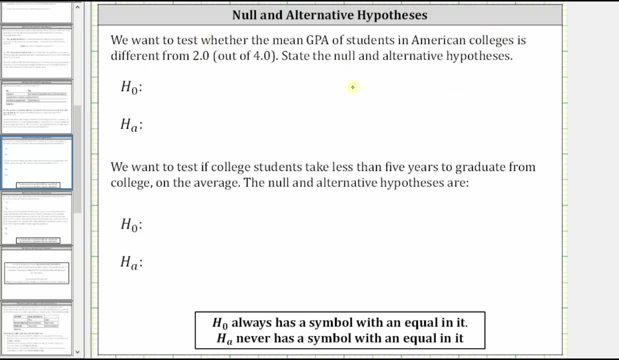 is different from 2.0, which would be mu not equal to two or 2.0. So if it's false that mu doesn't equal 2.0, then mu does equal 2.0. We know the alternative hypothesis. 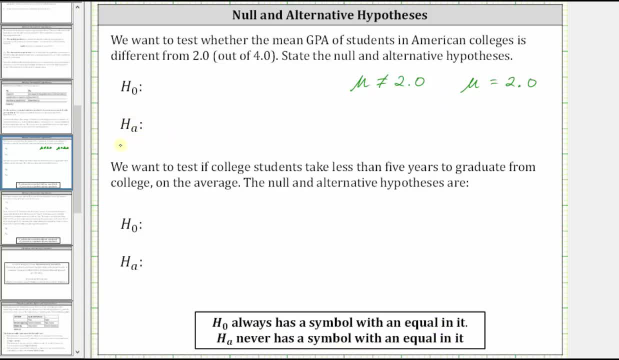 never has an equal symbol in it and therefore the alternative hypothesis must be mu not equal to two, which means the null hypothesis must be mu equals two And of course two and 2.0 are equivalent. Next we want to test if college students 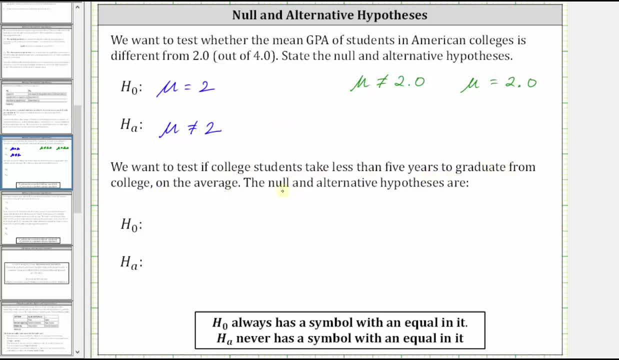 take less than five years to graduate from college on average. Again state the null and alternative hypotheses. So we're trying to test to see whether it takes less than five years, which would be mu less than five, And if mu isn't less than five, 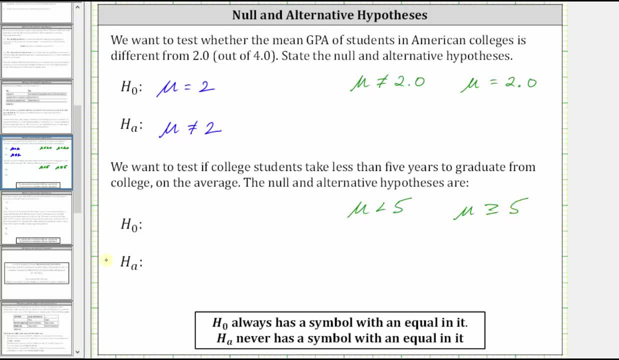 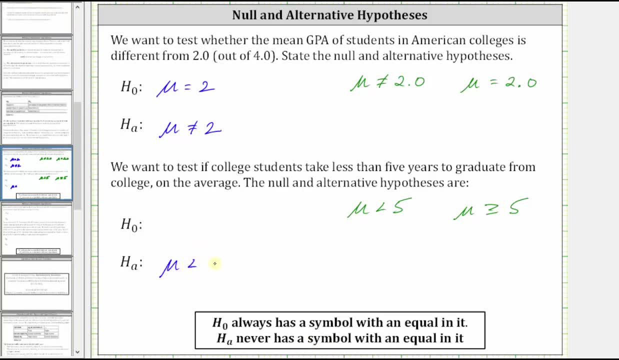 then mu is greater than or equal to five And again the alternative hypothesis does not have an equal symbol in it and therefore the alternative hypothesis is mu less than five and the null hypothesis does have an equal symbol and therefore the null hypothesis. 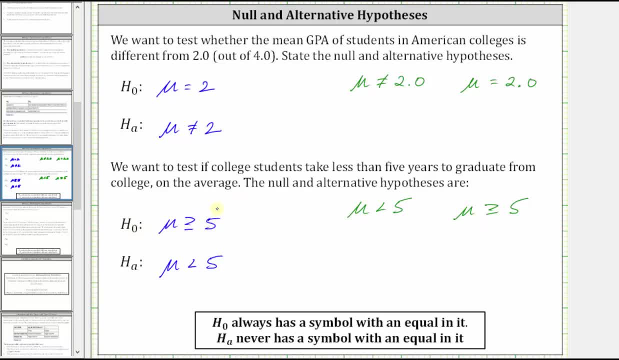 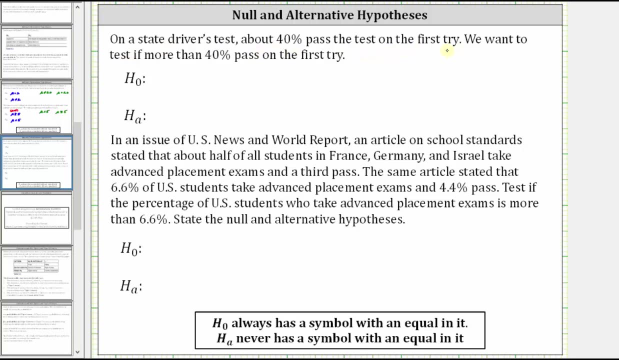 is mu greater than or equal to five? Just keep in mind some researchers would just state this as mu equals five. Next, on a driver's test, about 40% pass the test on the first try. We want to test if more than 40% pass on the first try. 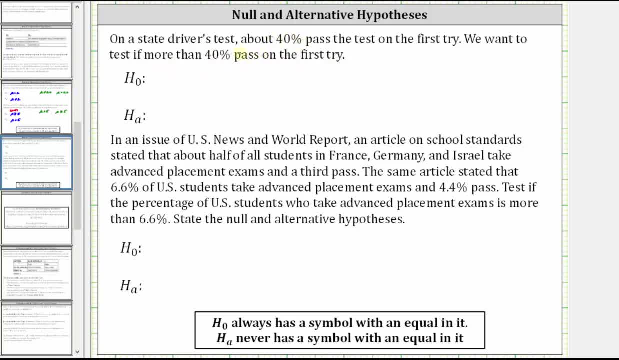 Because we have a percent here, where we use the variable p for the proportion we're testing to see if more than 40% pass, which would be p greater than 40% as a decimal is 0.4.. And if p is not greater than 0.4,, 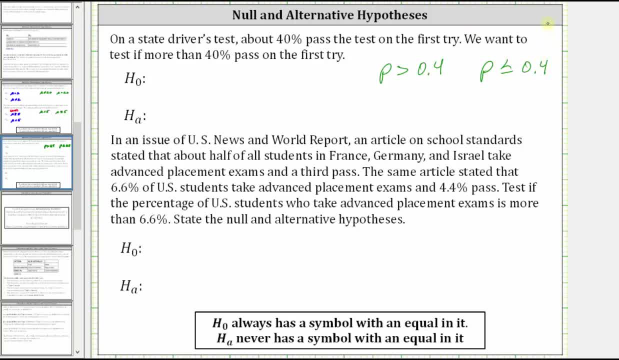 we would have p less than or equal to 0.4.. So, again, the alternative hypothesis does not have an equal symbol in it and therefore the alternative hypothesis is p greater than 0.4.. The null hypothesis does have the equal symbol in it. 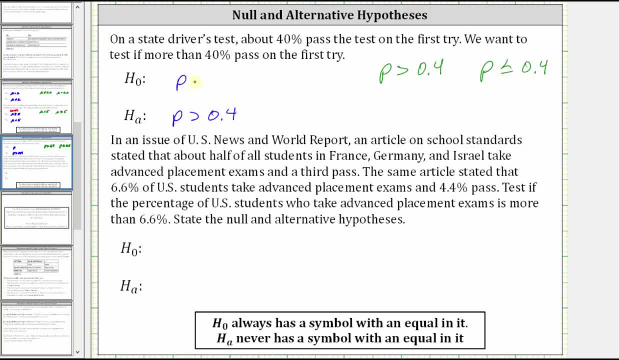 and therefore the null hypothesis is p less than or equal to 0.4, or, once again, some researchers would just state p equals 0.4.. And for the last example, in an issue of US News and World Report, an article on school standards stated: 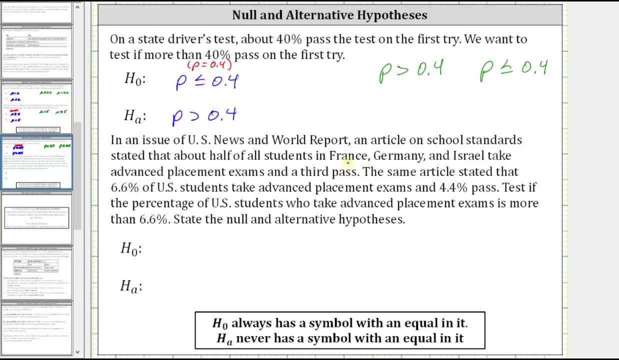 that about half of all students in France, Germany and Israel take advanced placement exams and a third pass. The same article stated that 6.6% of US students take advanced placement exams and 4.4% pass Test. if the percent of US students 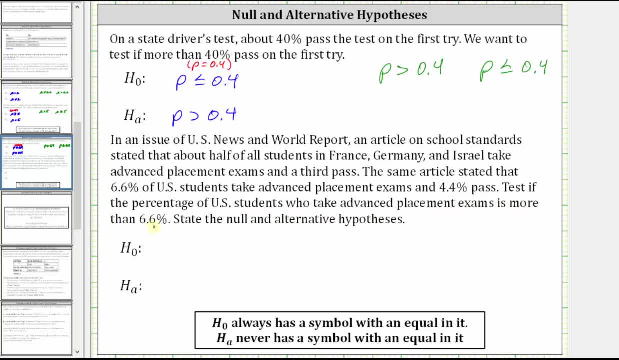 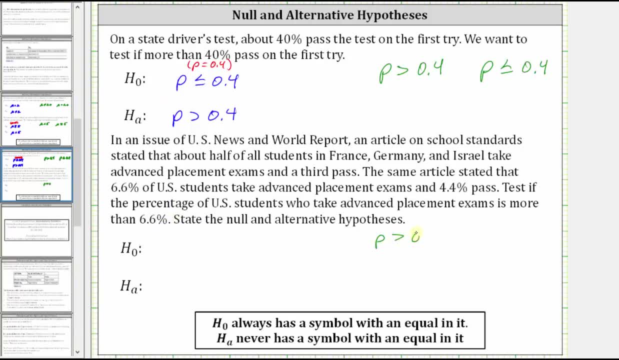 who take advanced placement exams is more than 6.6%. Well, more than 6.6% would be p greater than 0.066.. And if p is not greater than 0.066, p is less than or equal to 0.066..